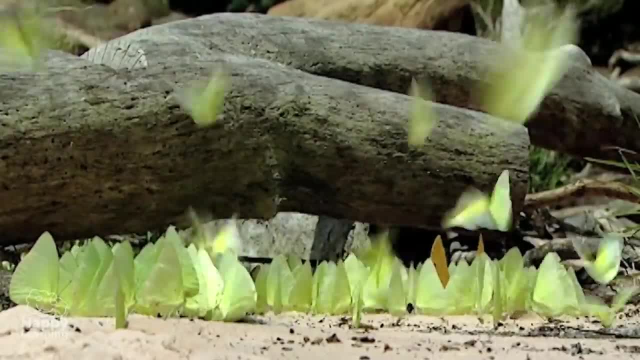 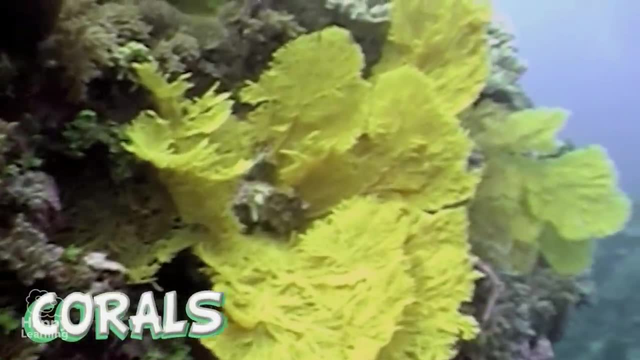 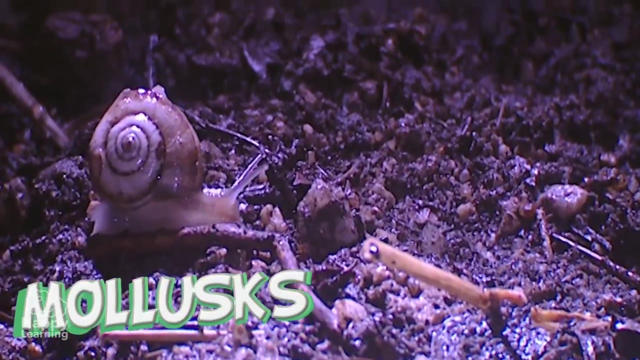 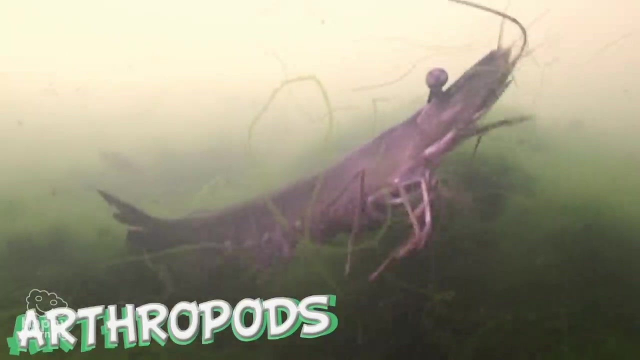 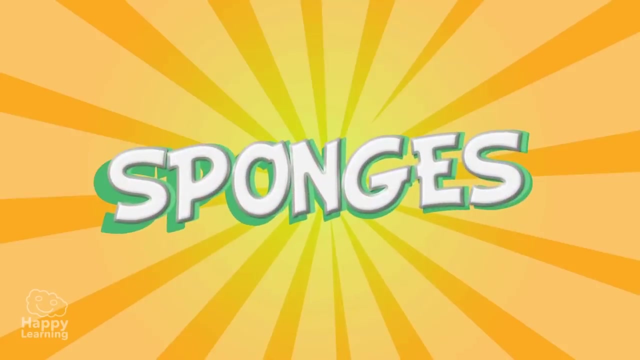 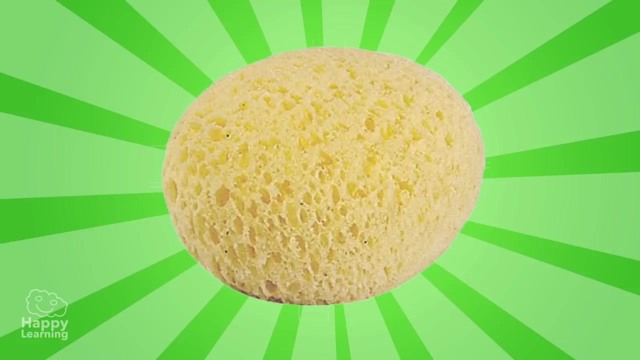 All the invertebrates are oviparous and we classify them in six big groups: Sponges, Jellyfish, Corals, Worms, Mollusks, Echinoderms and Arthropods. The sponges are aquatic animals that are shark shaped and the body is full of pores. 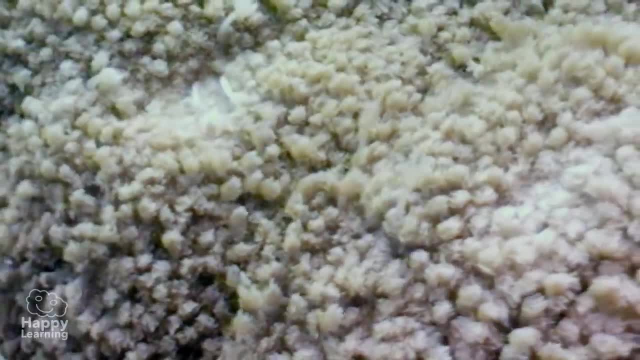 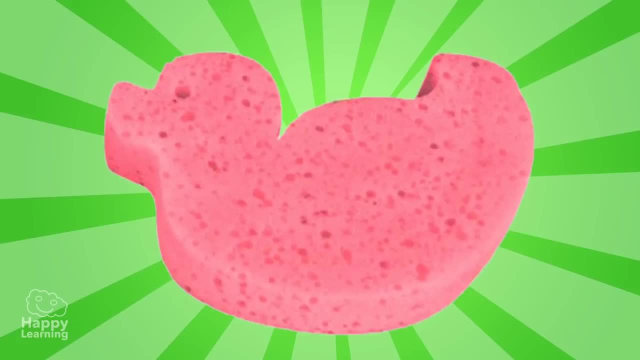 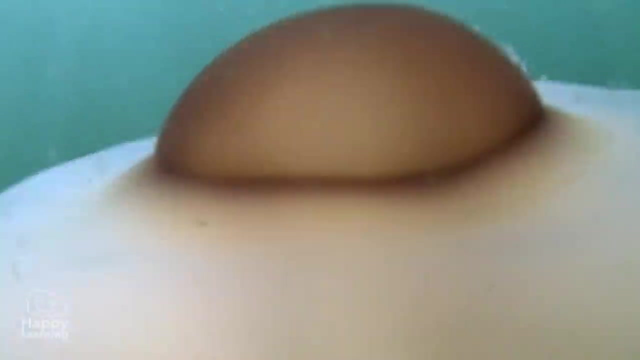 It is very easy to remember this group because many times we use them in the shower for personal hygiene. Yes, Many of the sponges we use in the shower are invertebrate animals. The jellyfish are invertebrate animals that live in the ocean. 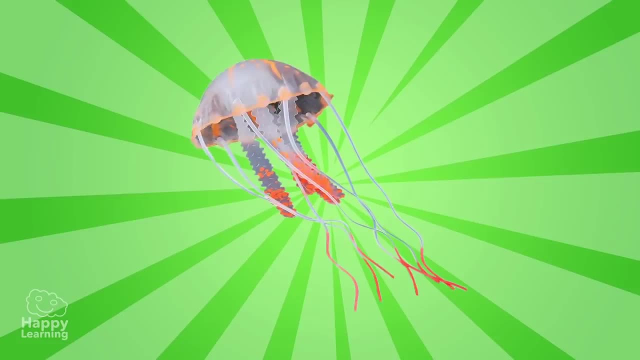 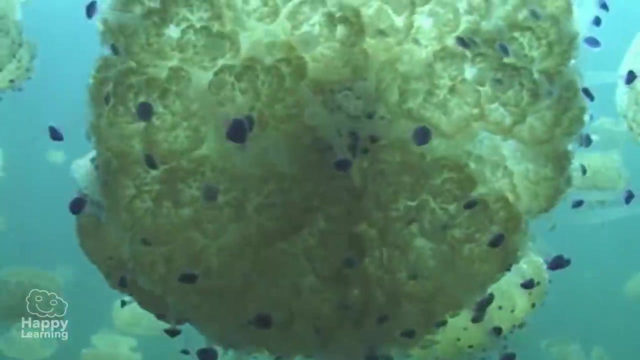 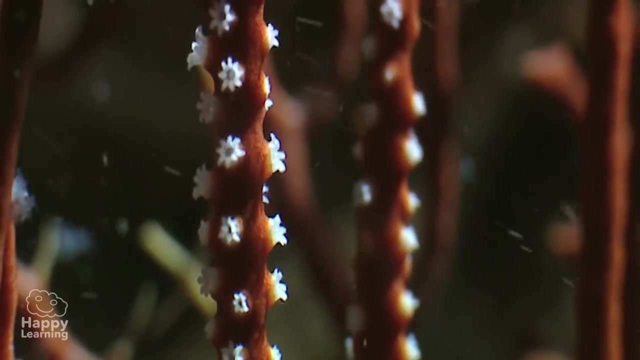 Their bodies are gelatinous and have tentacles. The truth is that when they appear in the beach, it is very annoying because their tentacles have small venomous stingers that produce very unpleasant bites. Corals are tiny marine animals that produce limestone residue. 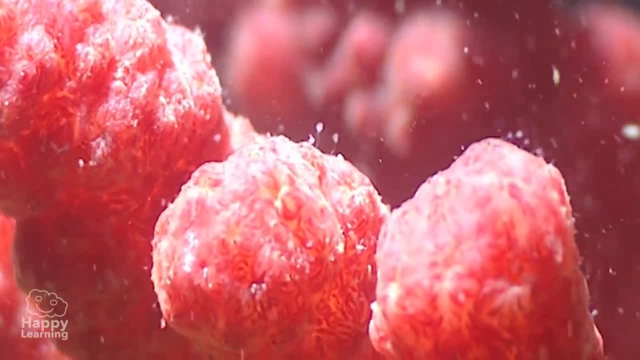 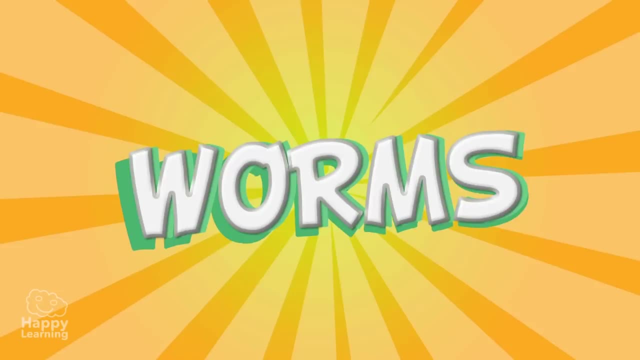 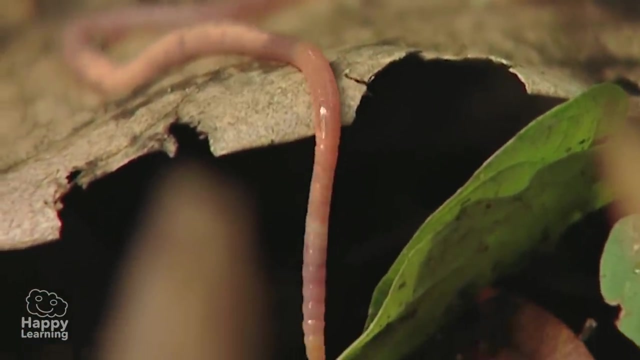 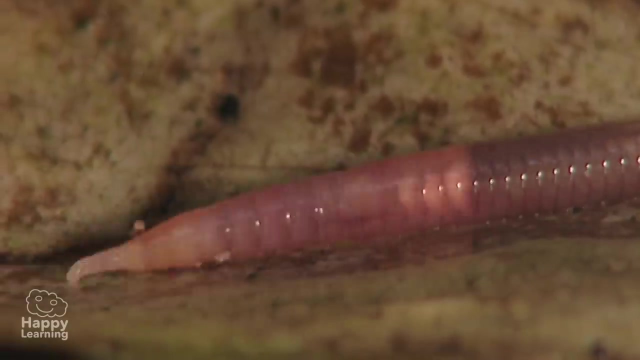 which give rise to beautiful shapes. Do you know this animal Exactly? It's a worm. Worms are soft and long invertebrate animals that move by dragging their body in the ground because they have no feet. They can be aquatic or terrestrial. 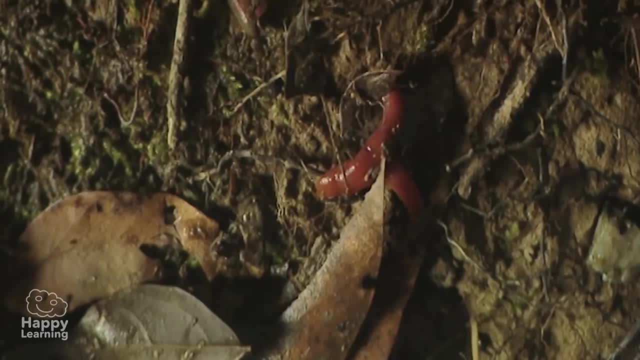 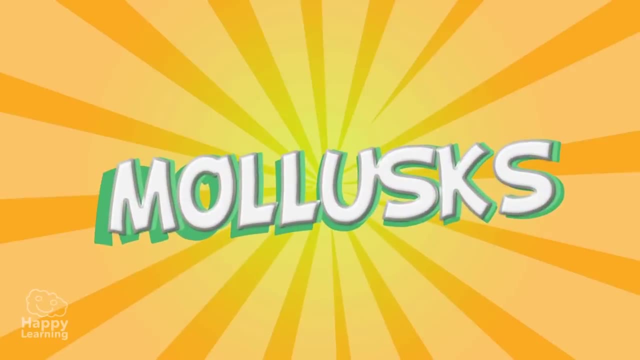 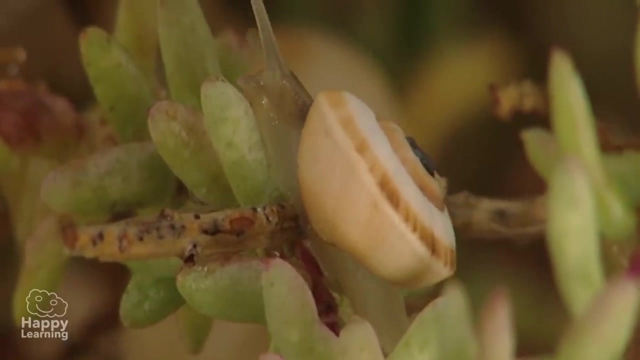 There are some worms that can be harmful, and that is why we must be careful with them. Can you see this snail? Well, snails form part of the mollusk group. The mollusks have a soft body without legs, and can also be aquatic or terrestrial. 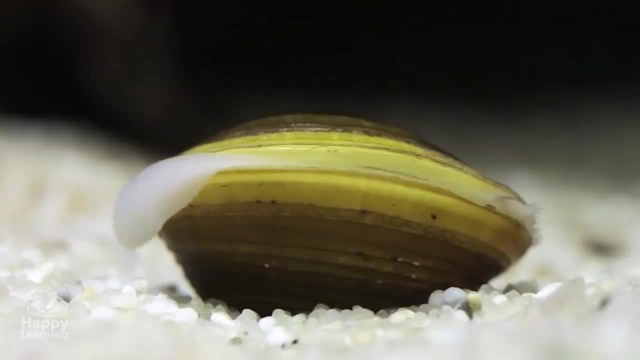 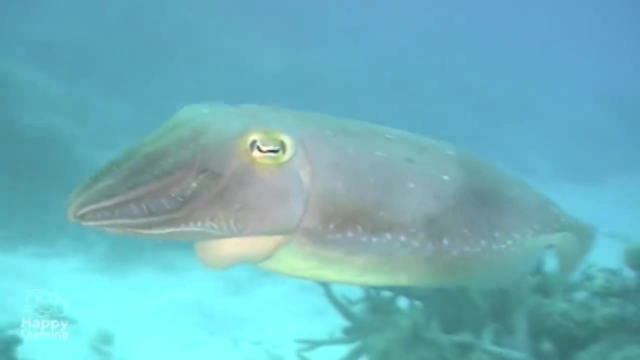 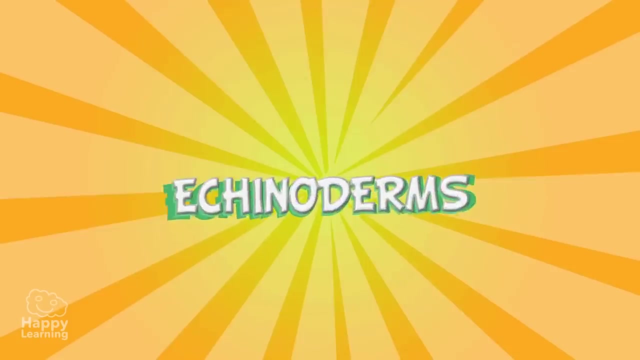 Some, like this snail, this clam and mussels, protect the body with shells, But there are other mollusks that don't have a shell to protect themselves, like slugs or octopuses. The Echinoderms are exclusively aquatic animals.